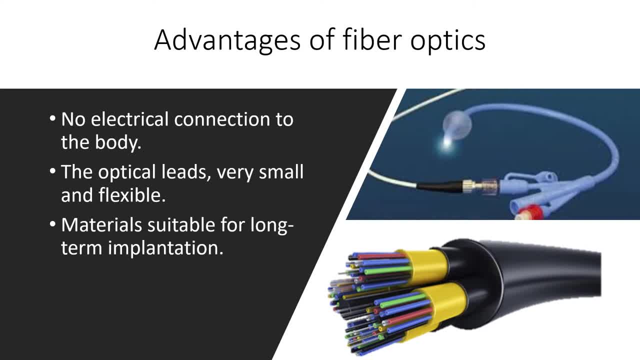 This is a great advantage, since, because of this, there is no chance of shocking a patient by mistake. Another big advantage is that the optical lids are very small and flexible. This allows doctors to use the devices on a small instrument, such as catheters, which are used to insert on the genital organs to drain urine. 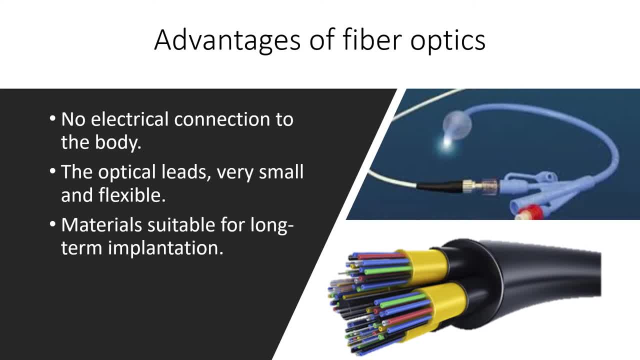 At the right of this slide there is a picture of one of these catheters. The small lids also help doctors to control the light. The small lids also help doctors to control the light. The small lids also help doctors to control the light. 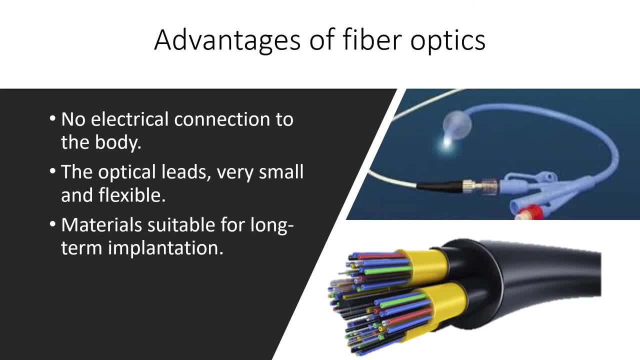 These are also used during close-body surgery to see when they are operating through a small camera and with a small flashlight. These are also used during close-body surgery to see when they are operating through a small camera and with a small flashlight. Fiber optic cables do not need any metal to work. 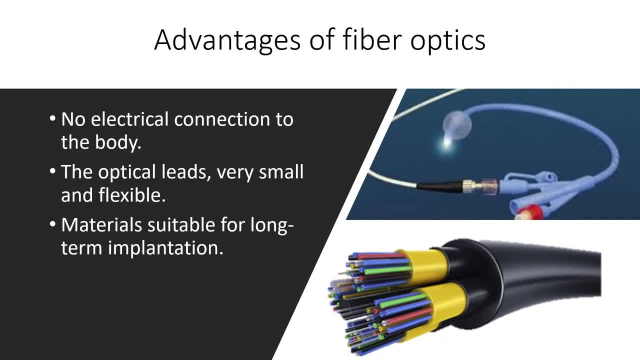 They can use plastic or silicone. they can use plastic or silicone, meaning that the materials would not oxidize or get any corrosion through time. This means that if an equipment was utilized during operation. utilized, it can be washed and disinfected for another use if handled with care, materials that 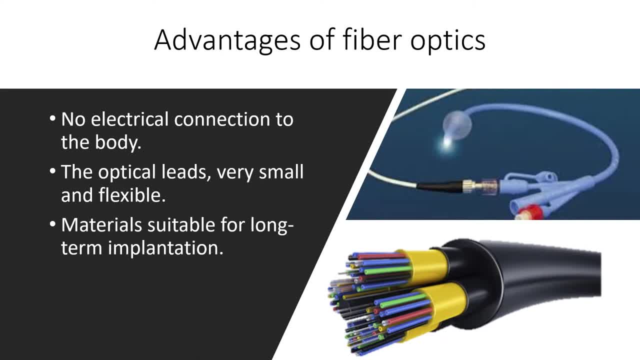 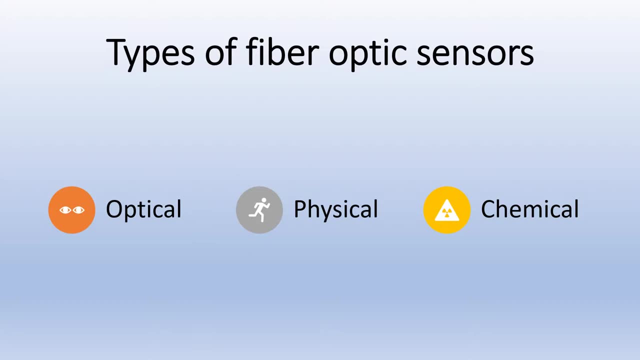 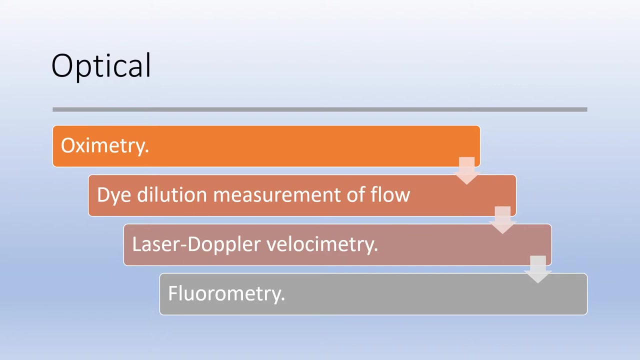 work with fiber optic cables will be able to last for a very long time. there are different types of sensors. today i will be explaining and giving an example of three of these types: optical, physical and chemical. an optical sensor is a device that usually detects light and, in sense, it's reading in an electrical form. 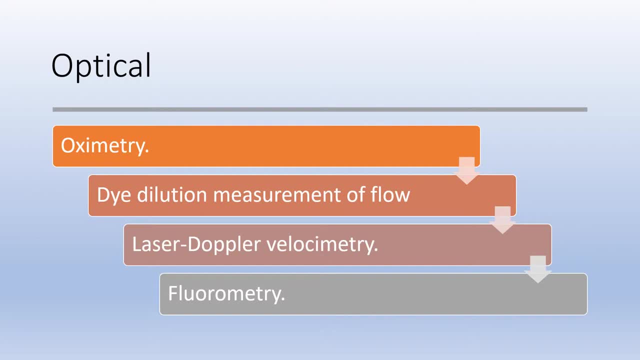 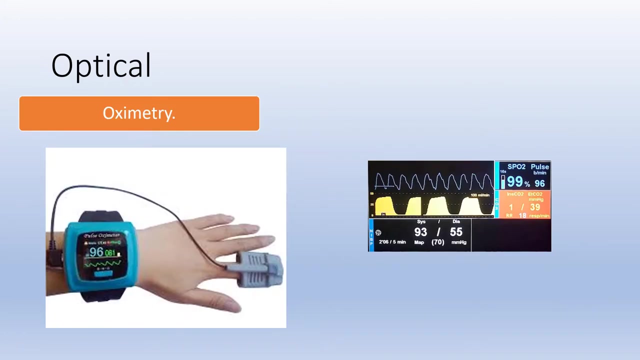 for medicine. several types of optical sensors exist: one of a symmetry, another diet, dilution, measurement of flow, then laser doppler, velocimetry and fluorometry as well. these are not the only ones. post-oxymetry is a test used to measure the oxygen level, or oxygen saturation of the blood. 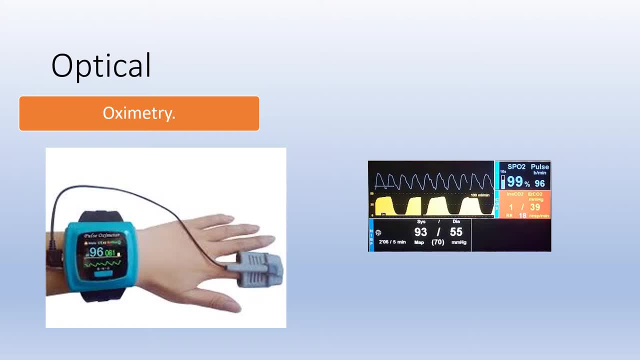 it is an easy, painless measure of how well oxygen is being sent to parts of your body furthest to your heart, such as the arms and legs. optical measurements of oxygen saturation depends on the difference in the absorption spectra of oxyhemoglobin and hemoglobin. optical fibers help in a case such as having an mri, because 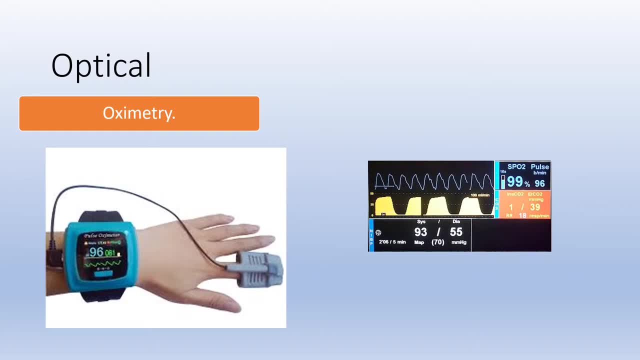 psychological monitoring during an mri is necessary to ensure the safety of patients when they are sedated, anesthetized or unstable. it helps in the case that no metal should be on the body when an mri is taking place. do not emit any noise on a study called monitoring heart rate and oxygen saturation with a fiber optic pulse oximeter. 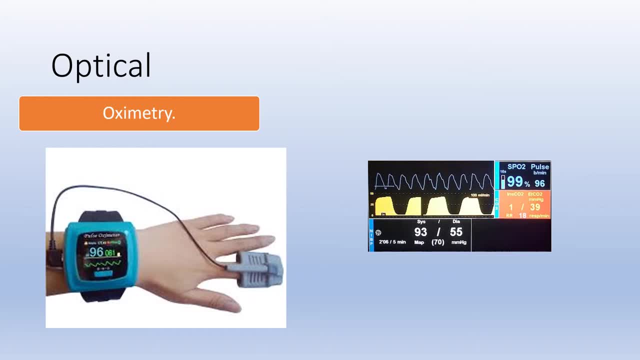 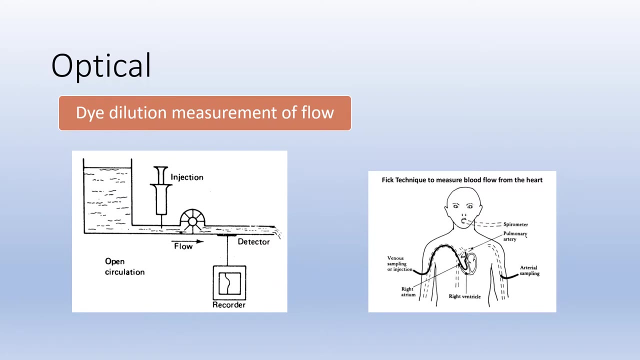 during mri imaging. they had a successful test using pulse oximetry during an mri. there was in 1984.. post-oxymetry, there is a method called dye dilution measurement of flow. it is used for measuring cardiac output, the same dual wavelength optics that are used to observe the concentration of injected dye in the blood. 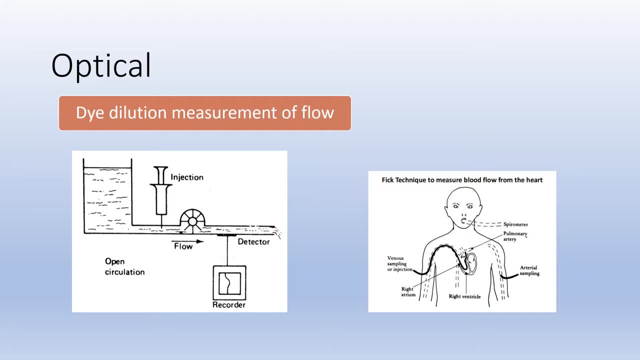 endocyanine green is commonly used. it has subsides strongly at 805 nanometers because there is a particular love of the possibility of largeIndustry absorption spectrum 2.. the study notes these differences aside from the last up-side down where we see that there was extrars sold in the 1960's. 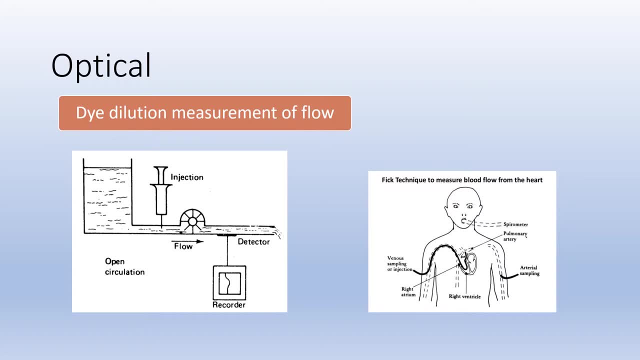 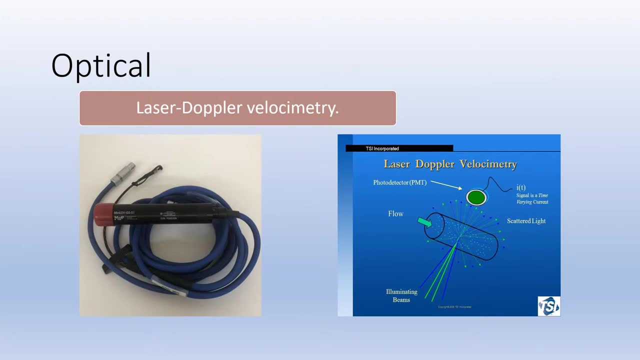 there is a conception technique that has been developed in recent years, for example, when Iranian in the 50s, drugs until the 90's, or also known as the laser Doppler anemometer is a type of interferometer who measures the velocity of objects using laser lens Coupling optical fibers. 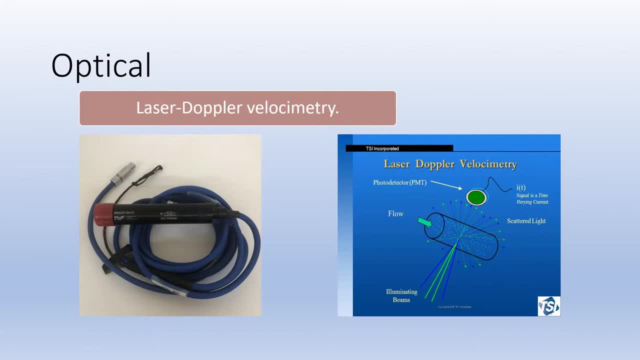 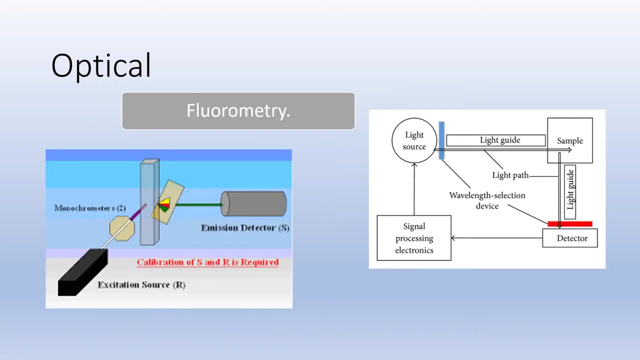 with the laser instrumentation allows the insertion of a fiber probe directly into blood vessels for observation of intraluminal velocity. A potentially useful application of direct fiber photometric is the observation tissue and blood luminescence Fluorometry is another type of optical sensing. 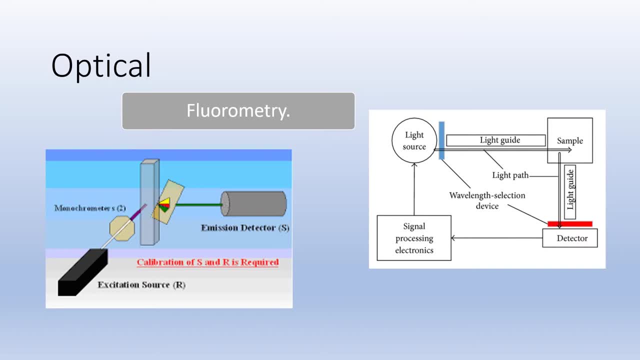 Fluorometry is an analytical technique for identifying and characterizing myniads of objects. Fluorometry is used to measure minute amounts of a substance by excitation of the substance with a beam of ultraviolet light and detection and measurement of the characteristic wavelength. 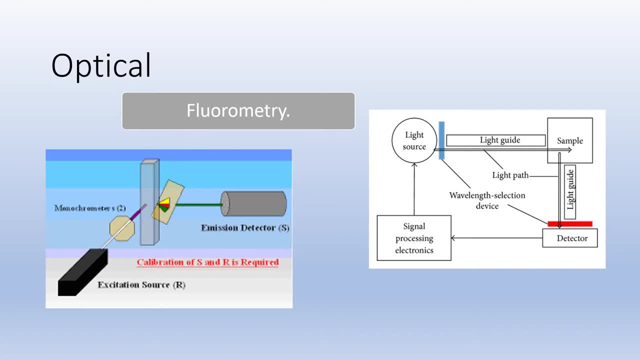 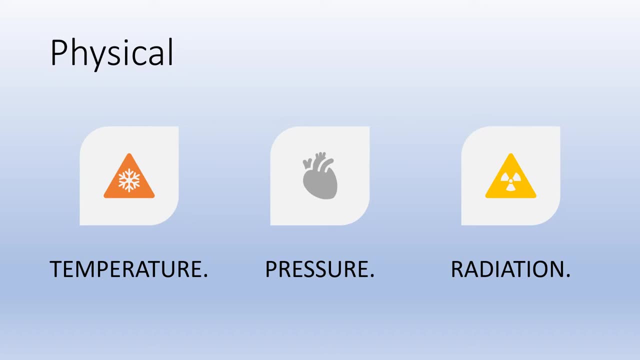 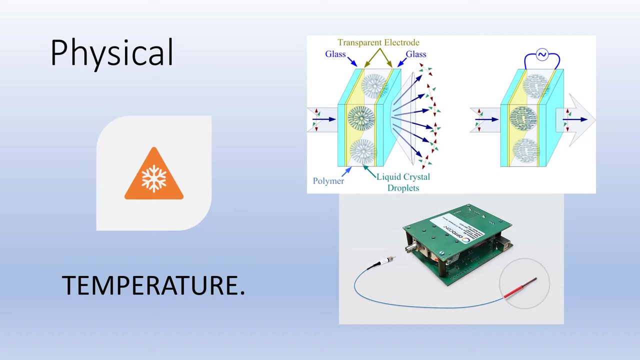 of the fluorescent light emitted. A more common sensor type is the physical sensor. For medical fields, they are mostly used to measure temperature, pressure and radiation. Today, we will be looking at temperature and the pressure types. The development of implantable temperature sensors is an important goal in medicine because 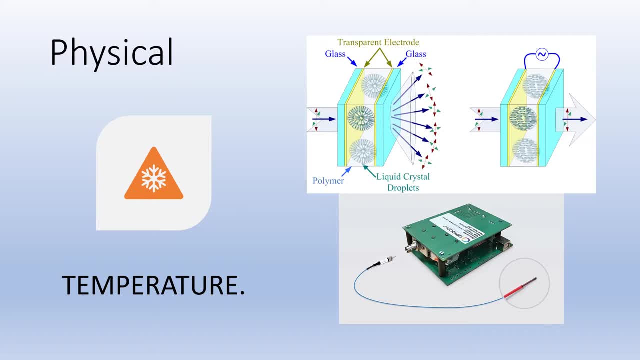 of the careful control of tissue heating required in the hyperthermal treatment of cancer. In order to reach this goal, the sensor and its leads will not interact with microwaves and will not be able to react to the temperature. Also, having the device at a small size is very important. Therefore, an optical sensor 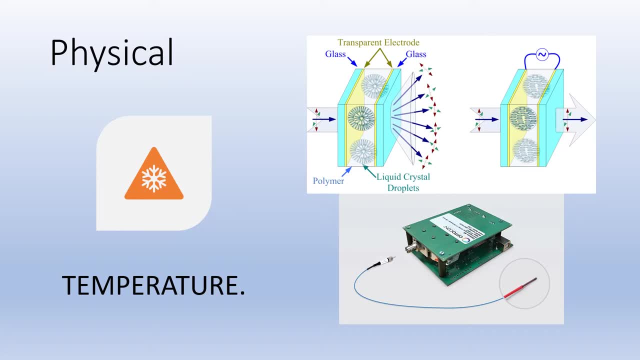 is ideal. One of the oldest and simplest types of temperature sensors consists of a layer of liquid crystals at the end of optical fibers. There is an example of how these liquid crystals work in one of these pictures. They are important because they have a variation of light at different temperatures. when a 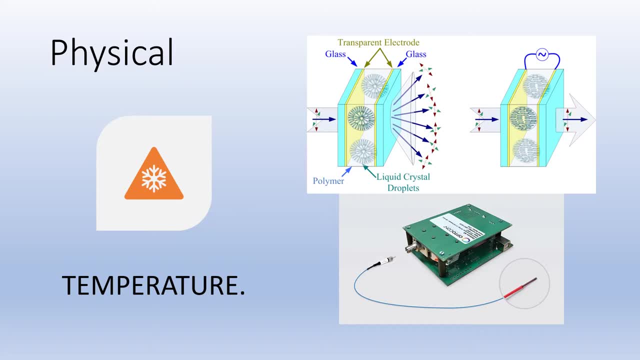 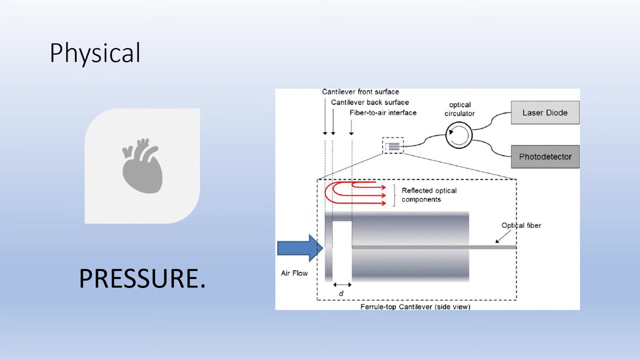 specific wavelength is disturbing it. An interesting application of liquid crystal thermometry was in a catheter for blood flow measurement by the thermodilution technique. A pressure fiber sensor works by using a cantilever mirror. This one is attached to a membrane located on the side of a probe. 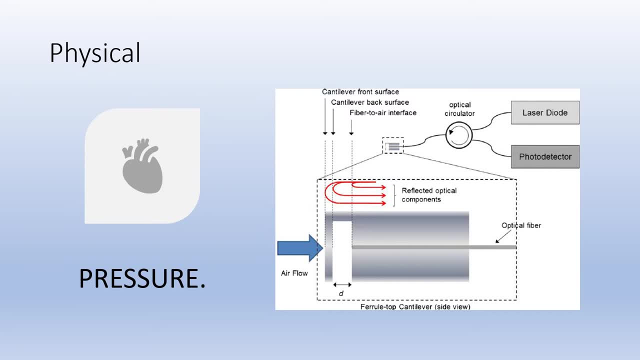 This one causes light to emit from a central optical fiber to be reflected differentially toward either two light-collecting fibers on each side of the central fiber, just as shown on this picture. The ratio of the light collected by the two apparent fibers is sent by the instrument. 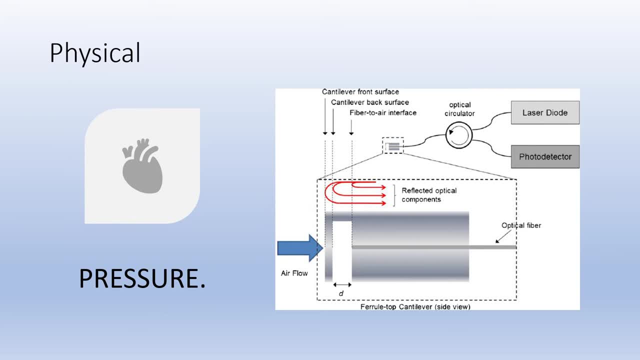 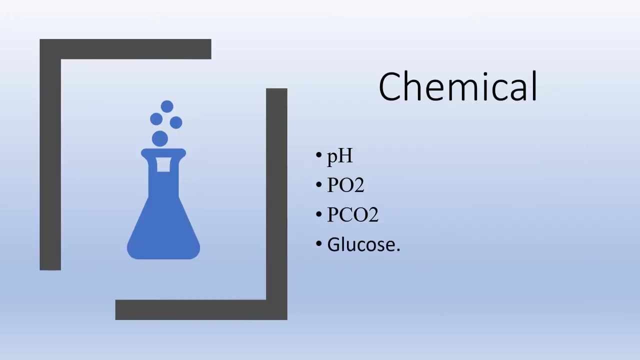 applying a feedback air pressure to the interior of the probe through a pneumatic connecting tube containing the optical fiber. With this knowledge, fiber optic transducers have been developed to monitor in granular and in cardride pressure. A very important application of fiber optics in medicine are the chemical sensors. 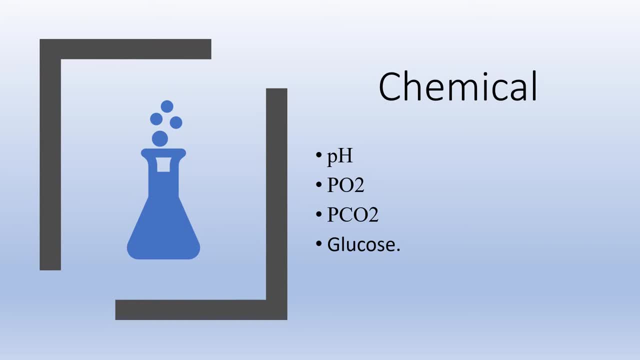 The basic idea of a chemical sensor is of an indicator packing in a permeable container at the end of a pair of optical fibers. The four listed components- pH, which determines the acidity, phosphorus oxide, carbon dioxide and glucose- are all measured with the same concept. 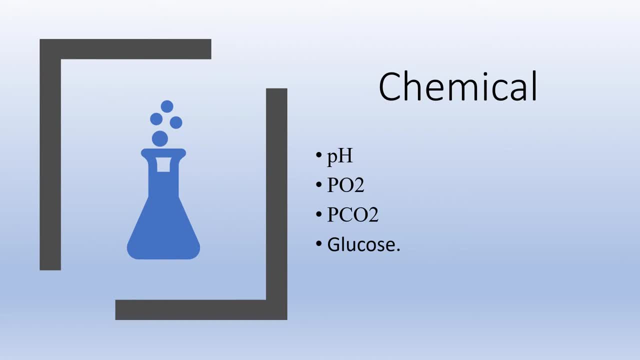 A specific dye is used for each one of them and, depending on the spectrum that they emit due to chemical reaction, is how much the person has on their bodies. This is an important sensor, since electrodes are not efficient enough to calculate chemical levels on the human body. 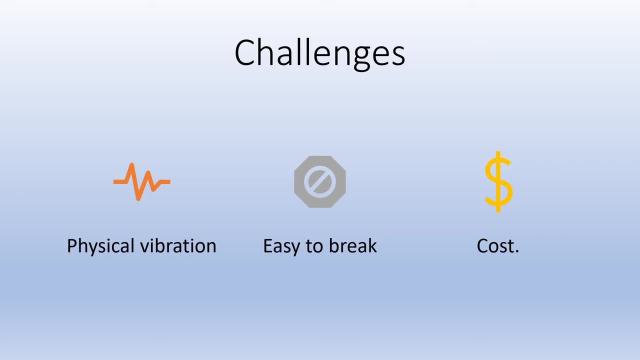 Just as everything has very good advantages and ways to make things better, there is always a cost or disadvantage that one has to deal with. However, optic cables are not an exception. One of these disadvantages is the physical efficiency. Vibration will show up as a signal for noise.